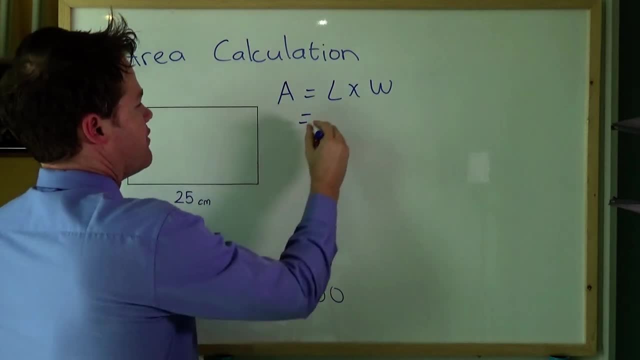 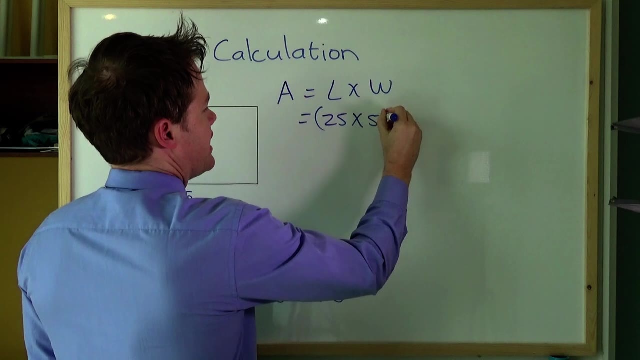 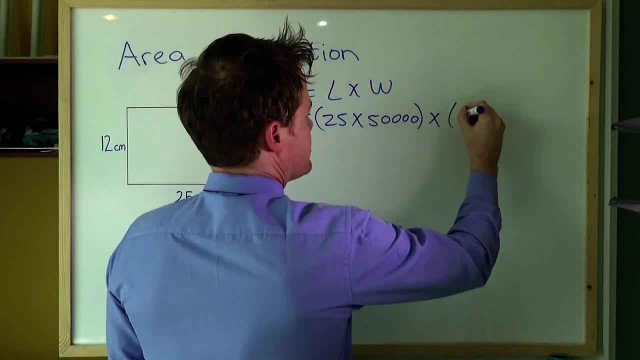 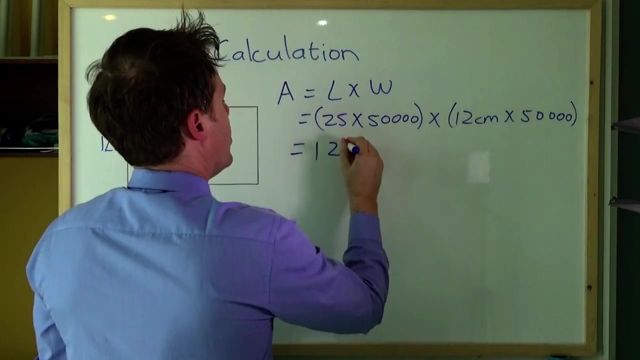 so the length is 25 centimeters, So we have to go 25 centimeters- I'm not going to write everything out- times the scale, which is 50,000.. And then the width is 12 centimeters times the scale, and this will give you 1,250,000. 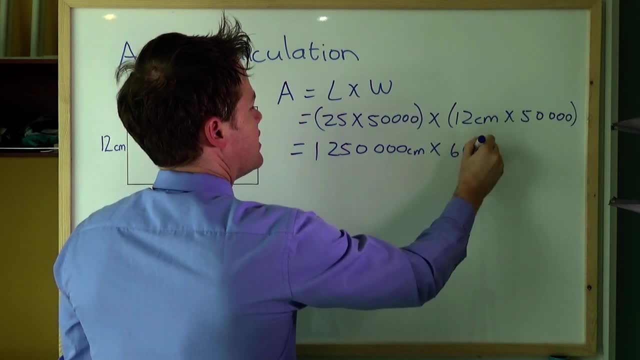 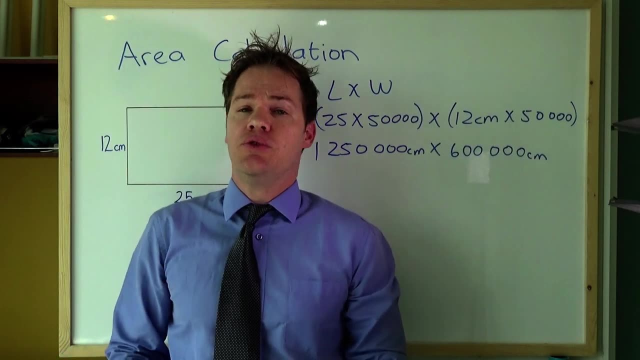 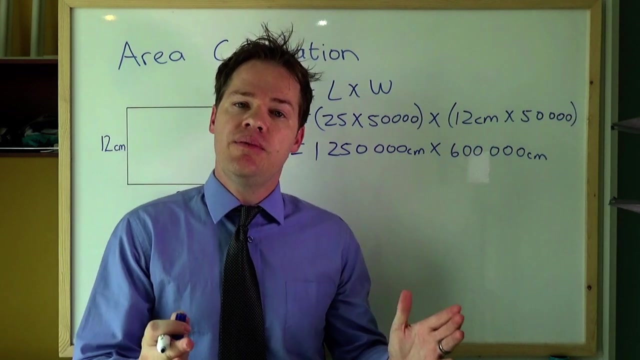 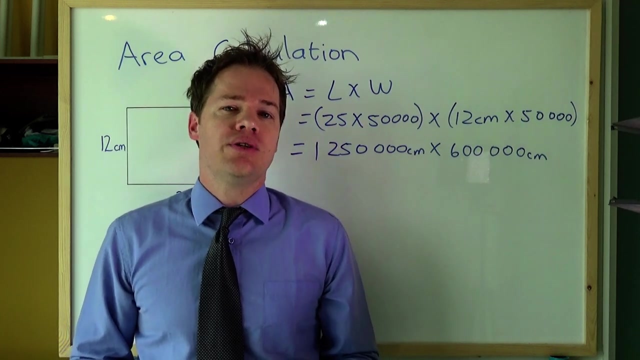 centimeters times 600,000 centimeters. Now, these numbers are very difficult to work with, so we are going to convert this to kilometers. Always remember: when we convert centimeters to kilometers, we say: divide by 100,000.. When we work with millimeters, though, we are going to divide by 1,000,000.. 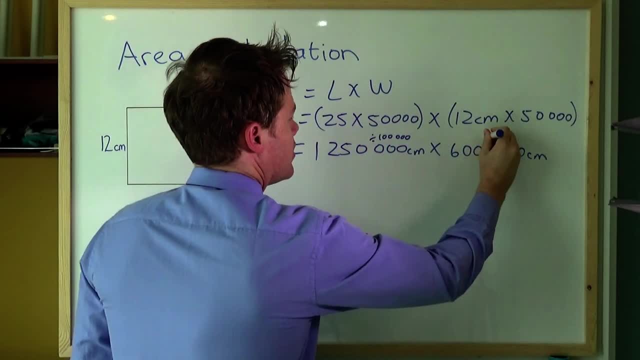 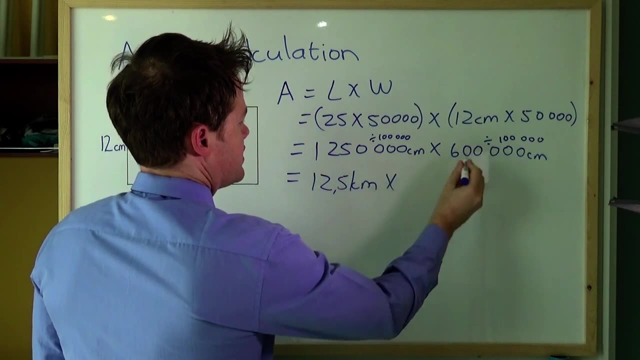 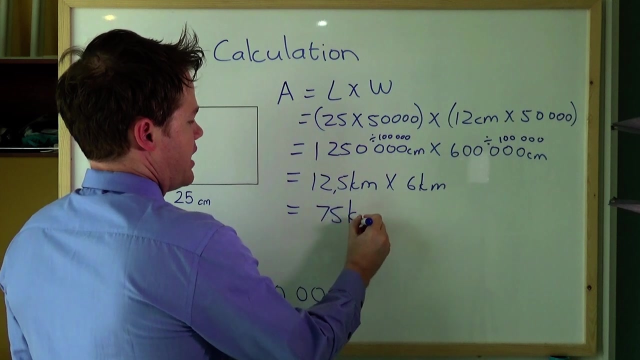 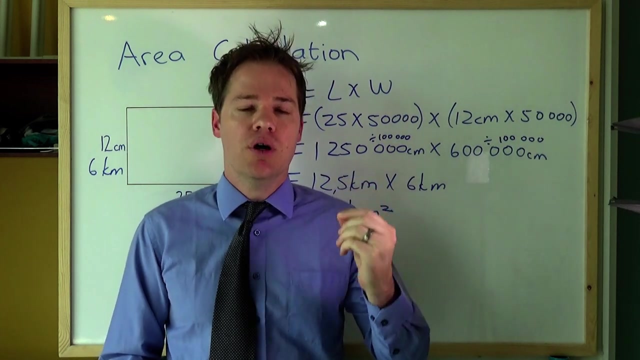 So let's see how it's done. So this is 12,5 kilometers times that's easy. 6 kilometers gives you 75 square kilometers. I always say things are a lot easier to remember if you understand how it works. Some people don't know what square kilometers are, so I'm going to explain this quickly. 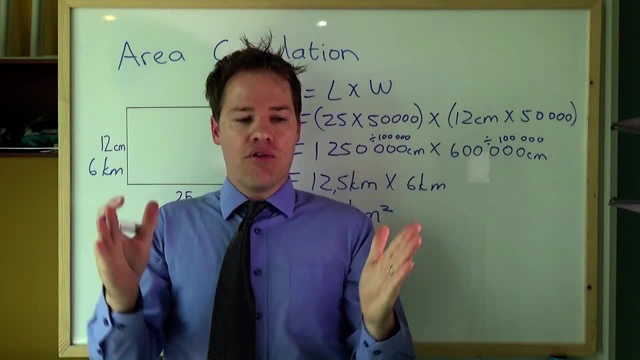 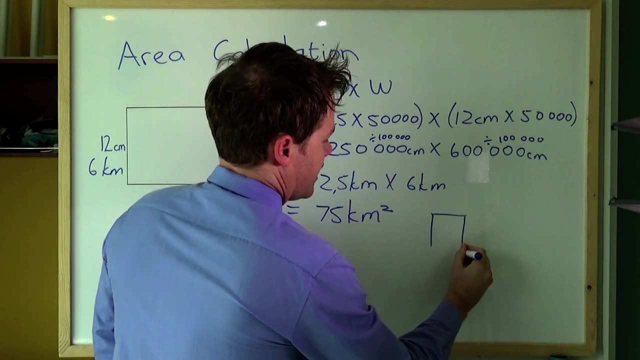 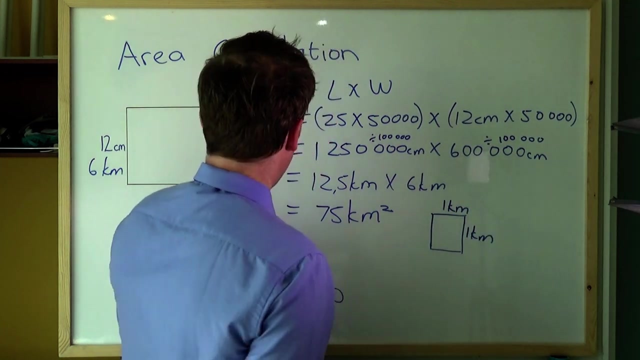 One square kilometer is a square of which each side is one kilometer long. so if this is a square kilometer right here, then each side of this square is one kilometer. So when we say that, if p goes below 10 km, it is 1 kilometer, if p goes below 10 km, it is 0.2.. 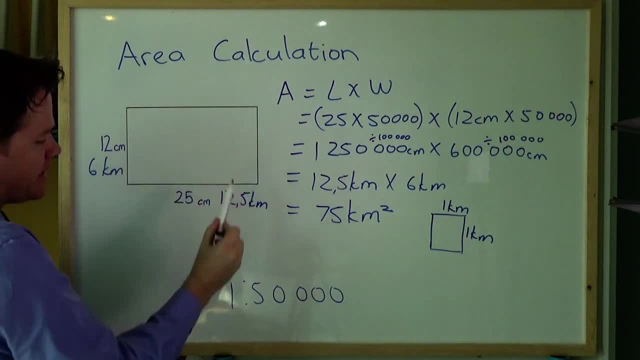 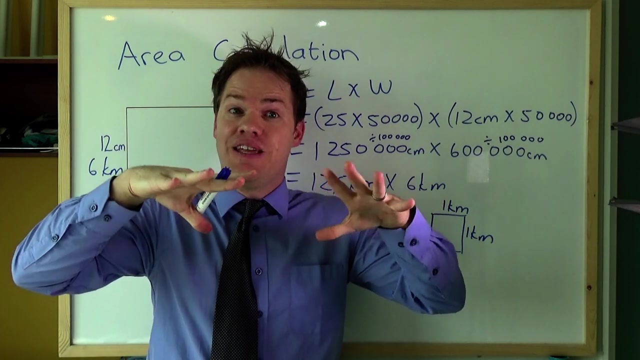 the area of this place here is 75 square kilometers, then it means 75 of these squares will fit into this area over here. How do you calculate the area when it's when the shape is irregular? and this is exactly what we are going to discuss in the next video. Thanks for watching. 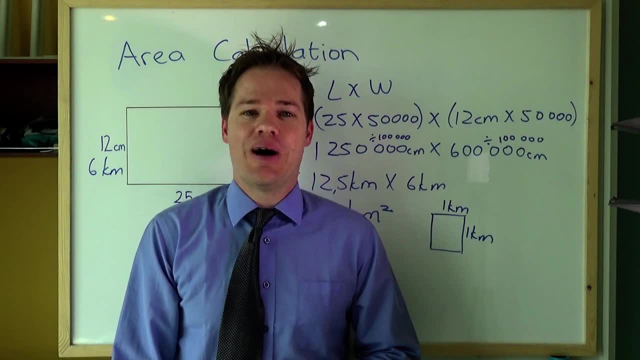 feel free to subscribe and see you next time. Goodbye.